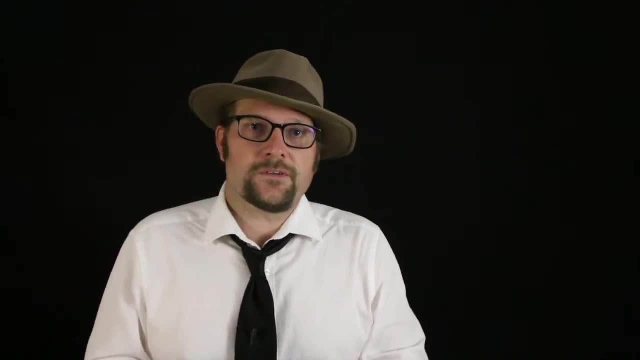 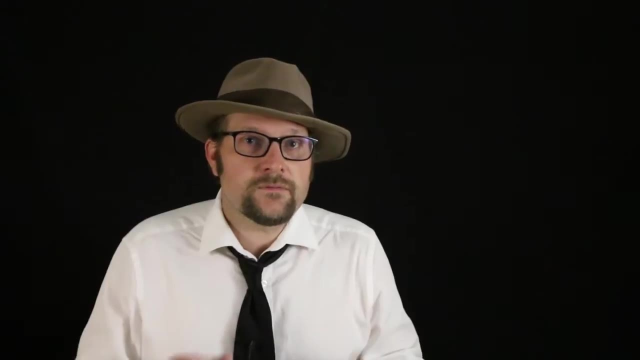 Welcome to Utah State University's Vertebrate Paleontology course. My name is Benjamin Brigger and in this lecture I want you to learn how to distinguish the unique traits found in the Multituberculates and their relationship to modern monotremes. 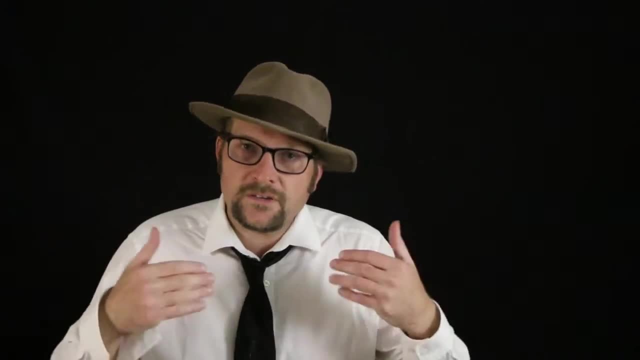 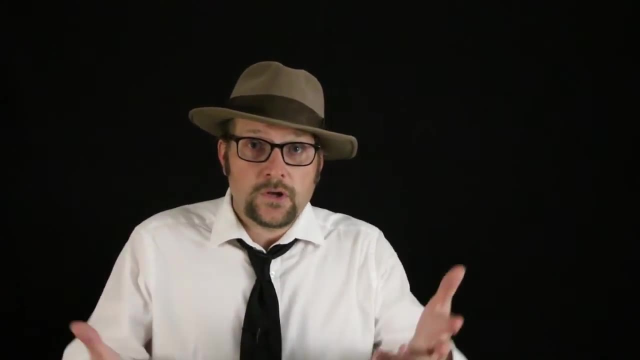 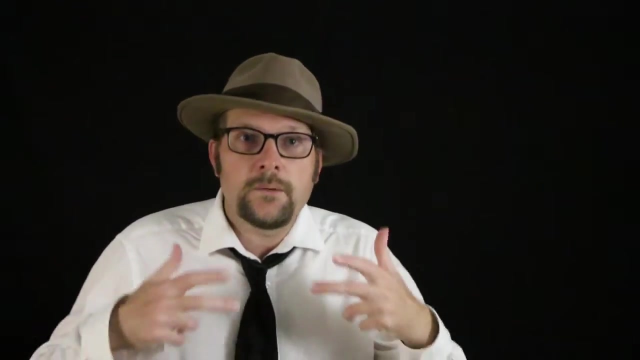 In doing so, we'll look at the two groups of successful mesozoic mammals and discuss the major evolutionary diversification of mammals during the age of dinosaurs. In the previous lecture we had discussed the anatomy of the first true mammal, Morganucodon. 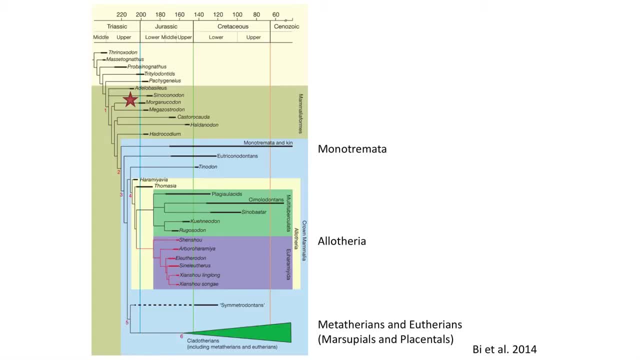 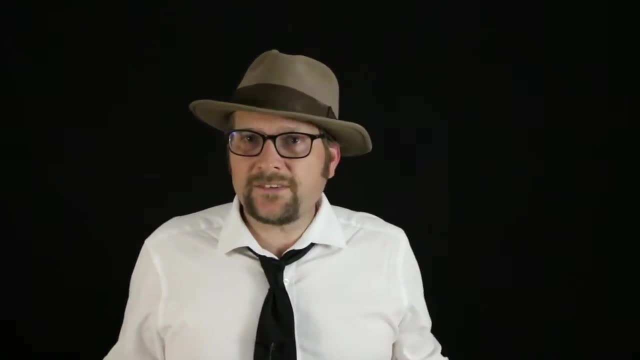 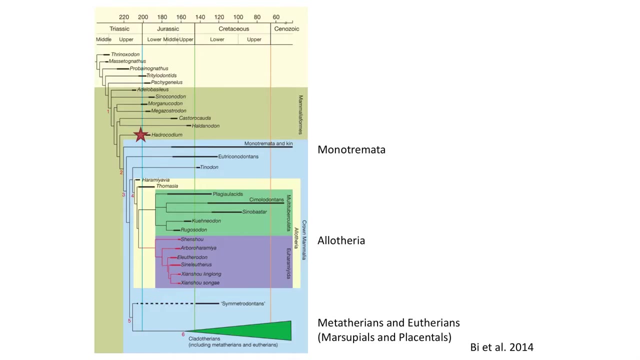 from the early Jurassic, as well as its close relative, the non-mammal Syconodon. During the late Triassic and early Jurassic, we begin to see the rise of the three major groups of mesozoic mammals: The Allia. Aetheria, the Monotremata and the late arrivers, the Metatheria and Eutherians, which start to appear in the Cretaceous. There are a few fossils known from the early to late Jurassic which preceded this split. These fossils are sometimes placed as early offshoots. from the three major groups of mesozoic mammals, and several of these miscellaneous mammals are at least worth mentioning. The first is a really tiny little fossil mammal, Hydrocodium, from the early Jurassic of China. The skull of Hydrocodium measures only 12 millimeters, which makes it one of the smallest. 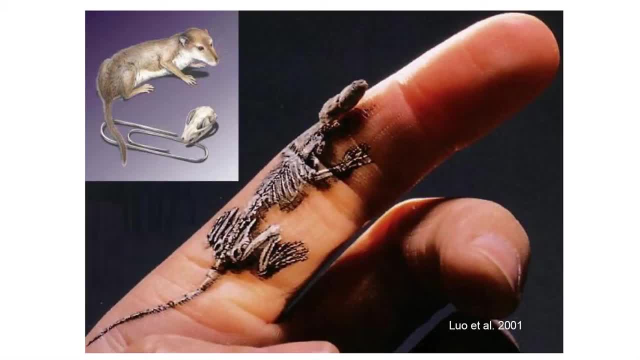 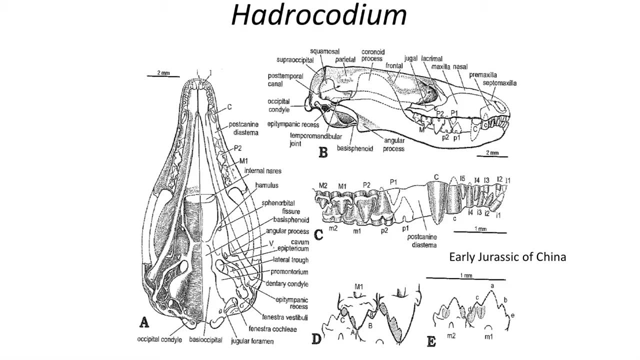 mammals ever known. Hydrocodium was about the size of a paper clip, But it is very important in understanding the evolution of mammals. Hydrocodium, like Morganucodon, is a true mammal. The ear and jaw resemble more advanced mammals and the teeth occlude with each other. 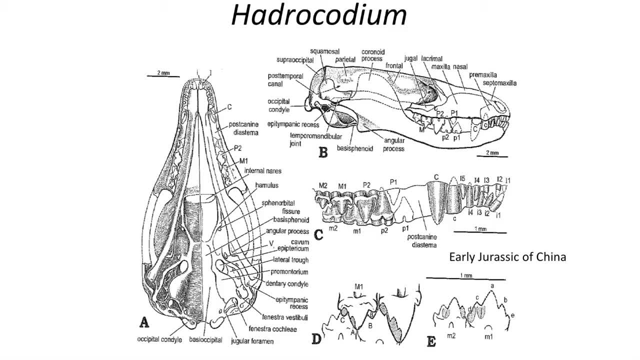 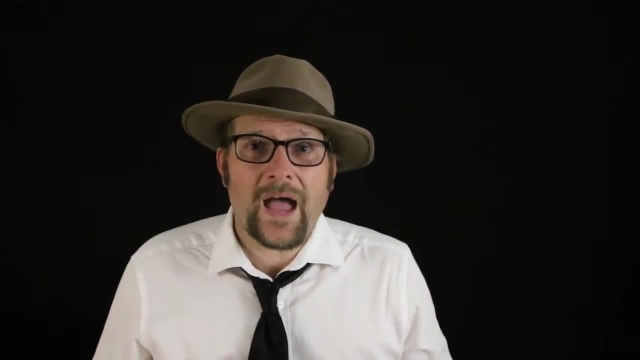 when the jaw is closed with distinct molars, premolars, canines and incisors. Its tiny size also was a feature of most mesozoic mammals, which would remain smaller than the size of a typical house cat for the next 130 million years. 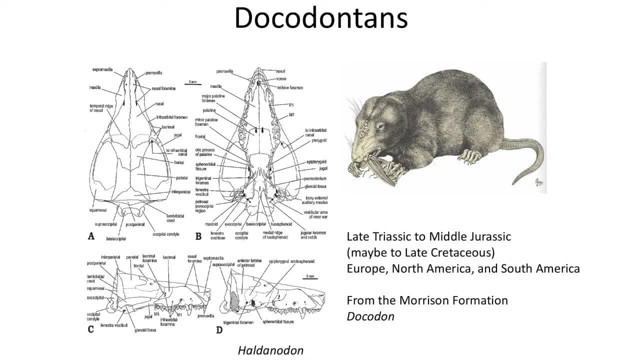 Another interesting mesozoic mammal group that appears to split off before the trification of mesozoic mammals is the Docodonts. Docodonts are a small group of very rare fossils that are found in the late Jurassic from the same rock units that produce. 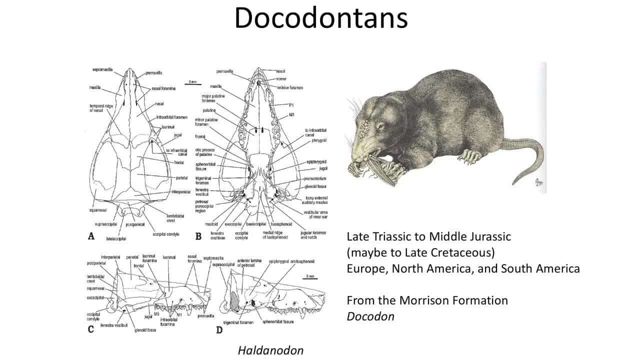 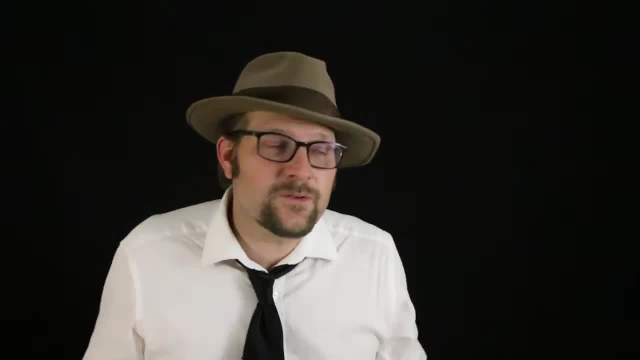 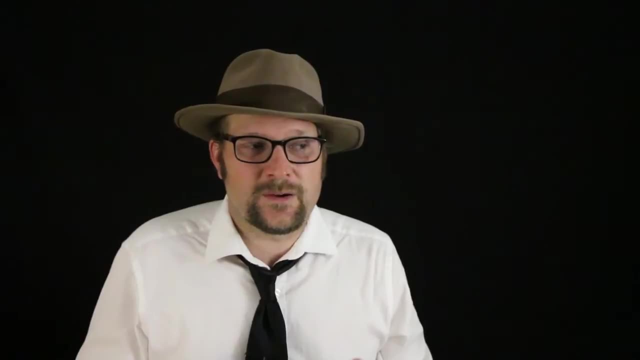 giant dinosaurs. Apatosaurus and Diplodocus Docodonts are small mole-like mammals which are very rare. My dream is to find one of these tiny little fossil mammals, but so far I have not found one in the Morrison Formation, despite all my looking. 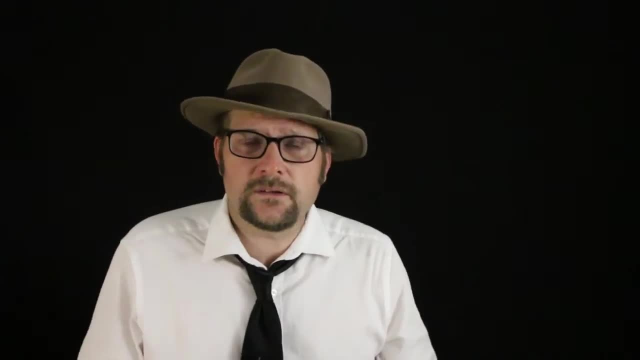 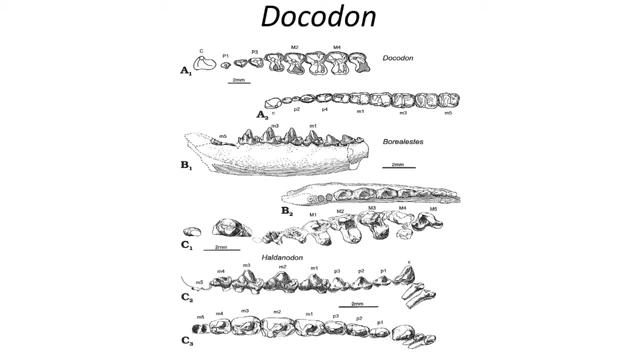 Fossils are rarely found, but over the years a nice record has slowly emerged. The Docodonts are recognized by an unusual pattern of cusps and basins on their teeth and the hourglass shape of their upper molars. Because these early groups are outside of the branch that includes all living, mammals. they are sometimes grouped together in a more broad group than just mammalia called the Mammalia formis. The first of the three groups, the Allotheria, are recognized in the fossil record clear back to the late Triassic, but they quickly radiated during the Jurassic. 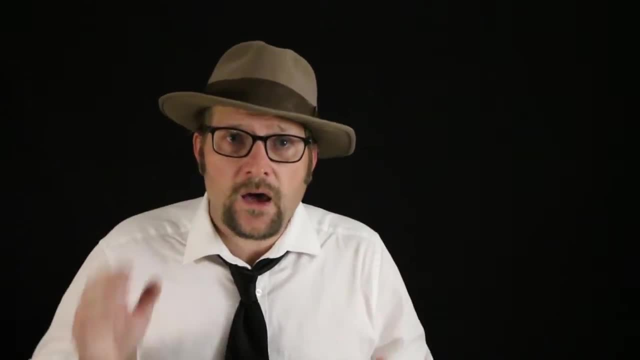 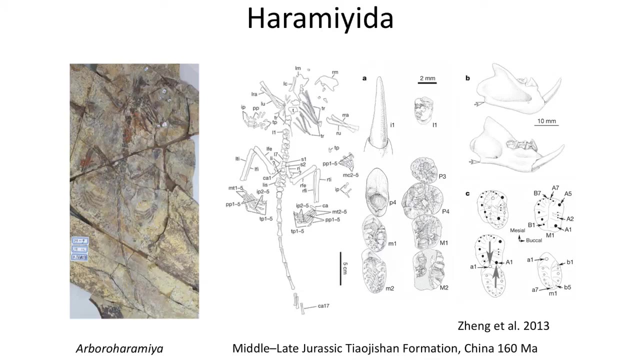 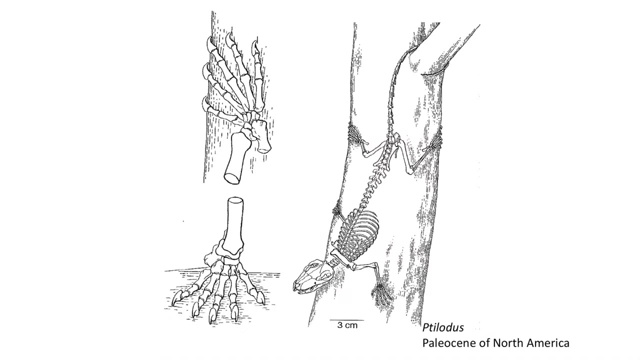 and Cretaceous, becoming one of the most dominant of the Mesozoic mammalian groups. The most primitive group is called the Hyromibiidae, with later forms in the Jurassic that split into two subgroups: the Euhydromidiidae and the Multituberculata. 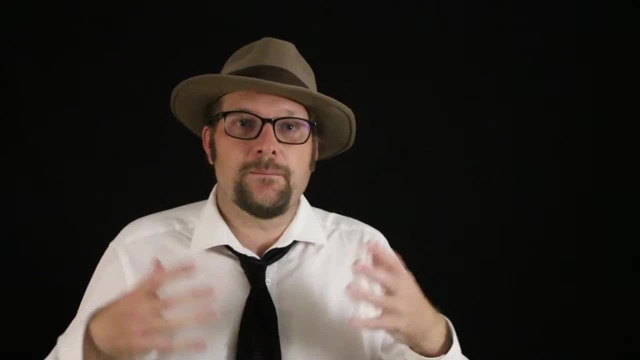 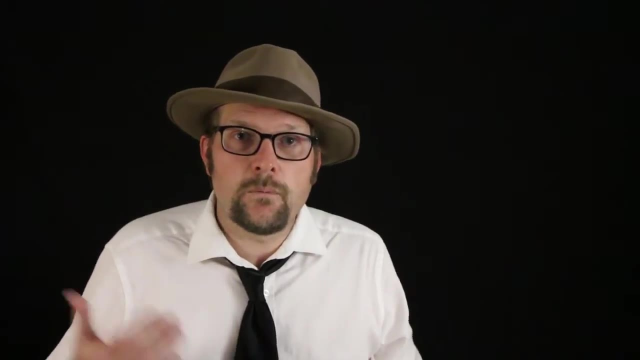 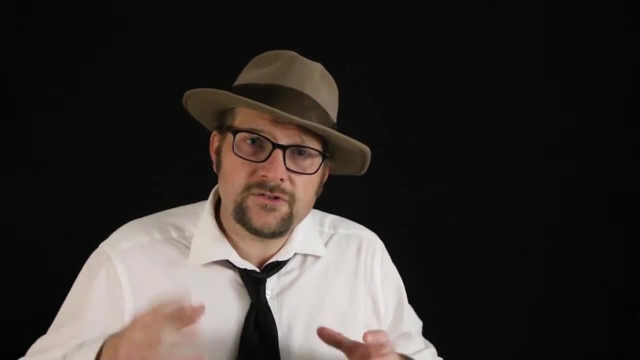 There is some debate whether the two groups are a monophyletic, as some people have suggested that the Euhydromibiidae are a much more primitive branch on the Mammalian tree. However, there are two major characters that they all have in common. 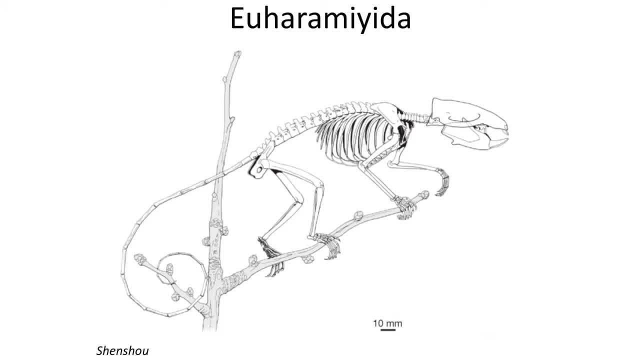 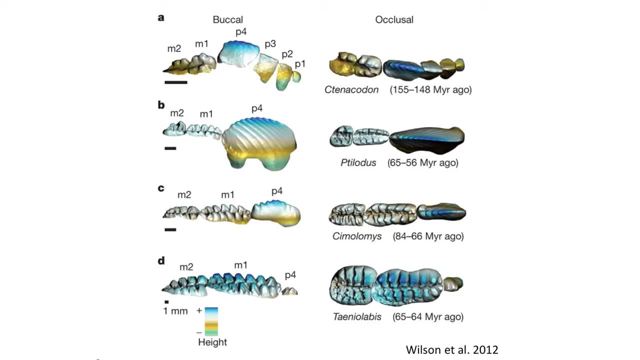 All members of the Allotheria have large incisor-like teeth and multicuspid molars which feature rows of cusps. Most of the Allotheria have large incisor-like teeth and multicuspid molars which feature rows of cusps. Most are. 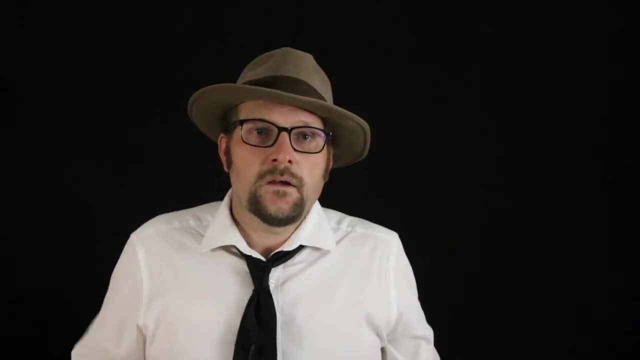 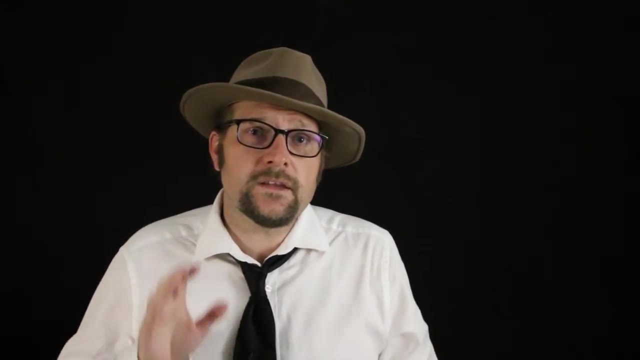 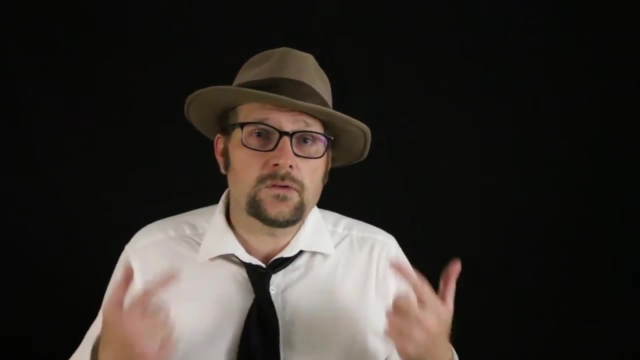 arboreal mammals and some burrowers, But they likely developed these very specialized teeth to feed on seeds. During the Jurassic, seeds were restricted to the Gynneosperms, including primitive Ginko and Conifers. The long incisors allow these animals to 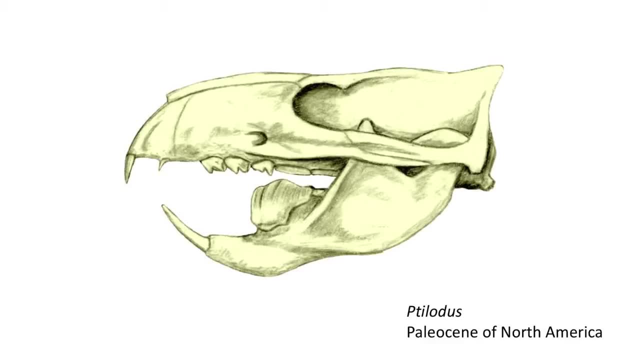 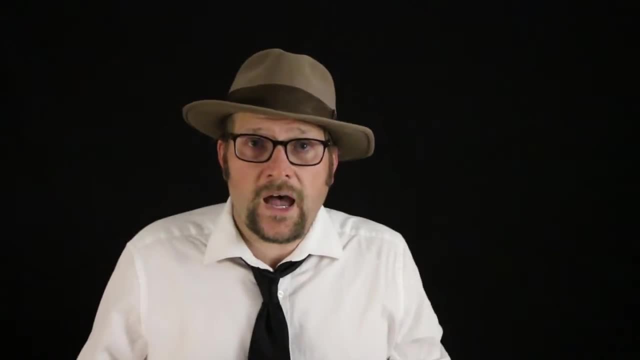 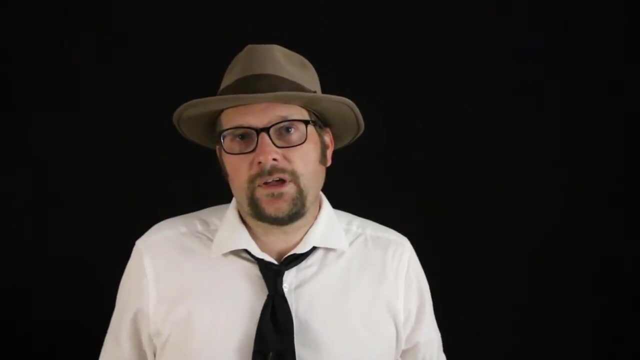 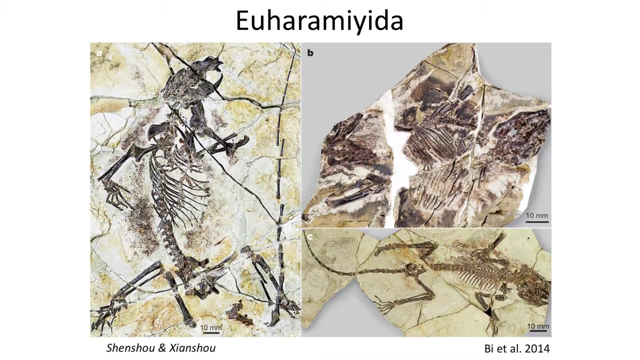 pluck out seeds from cones and use their multicussed cheek teeth to crush up the pulp. Several of the early Hyromimiidae and Euhydromimiidae fossils are known from nearly complete fossil skeletons from China, including Arbiohyromimiidae, Shi Shu and Xingshu Sha, all from the Jurassic. 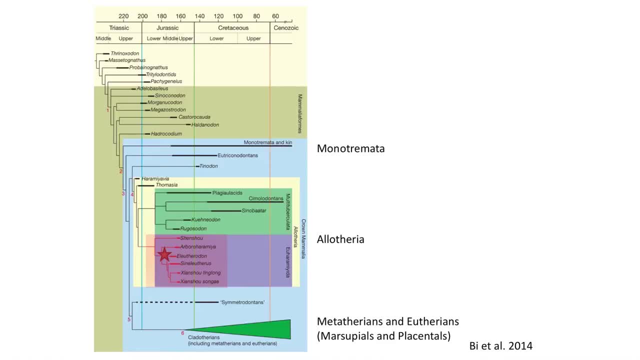 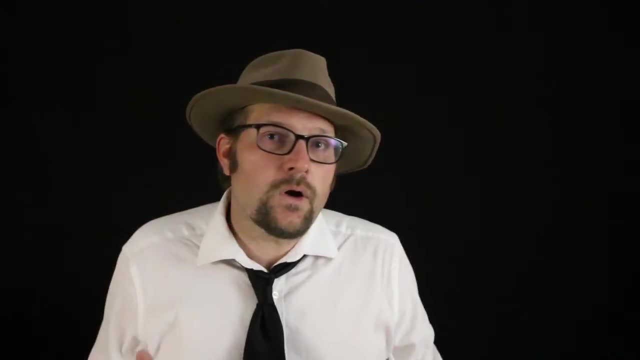 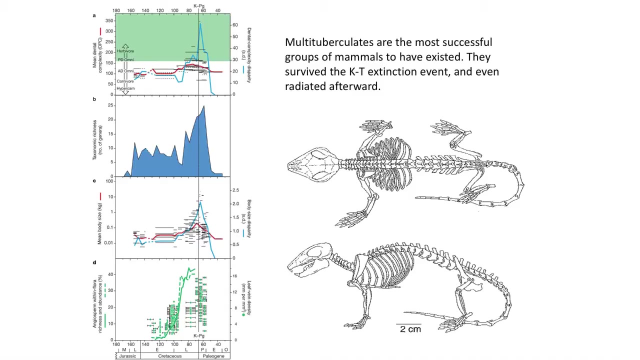 And in fact the Euhydromimiidae are restricted to the Jurassic period. The Group of Alatheria, the multi-tuberculates, would go on to success in the Cretaceous and the Cenozoic. The multi-tuberculates get their name from the many cuffs that form rows on their molar-like 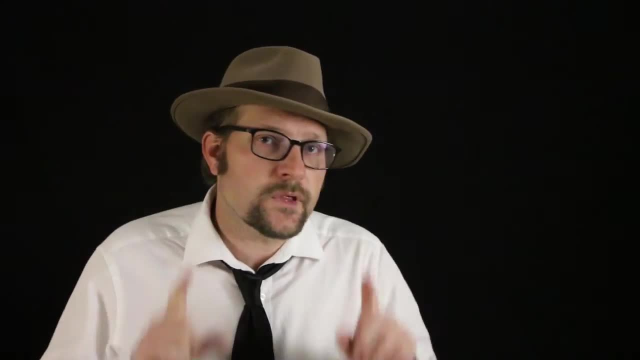 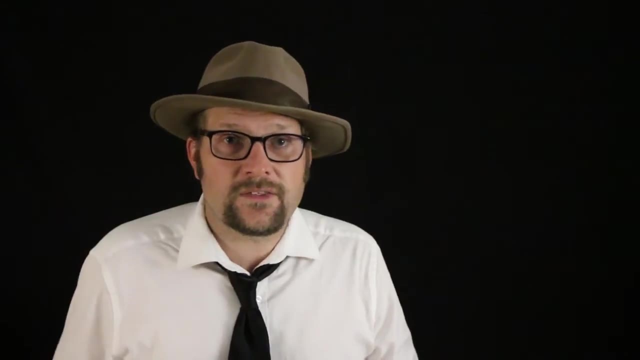 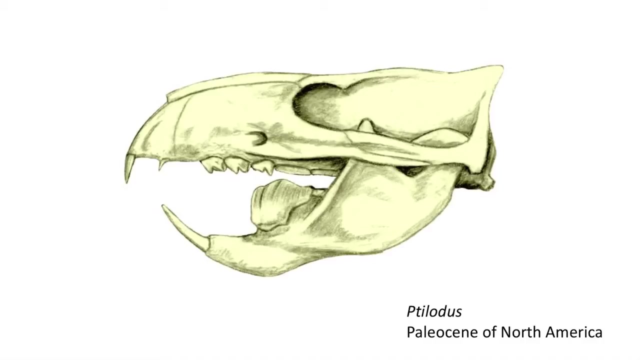 teeth. The multi-tuberculates also developed something quite unique: a blade like fourth blower premolar, which was used to to slice the huss of seeds of the Female. Thank you, Thank You, and nuts. This innovation led to great success for the group with the origin of angiosperms. 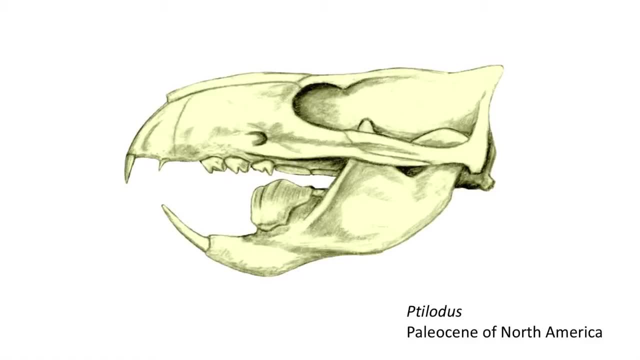 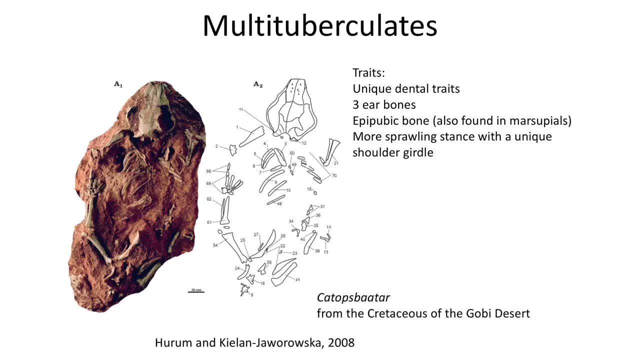 the fruiting and nut-bearing plants that first appeared in the early Cretaceous- The early Cretaceous of Mongolia. the multi-tuberculates also became excellent burrowing animals, and a number of complete skeletons are known from the same rock units. 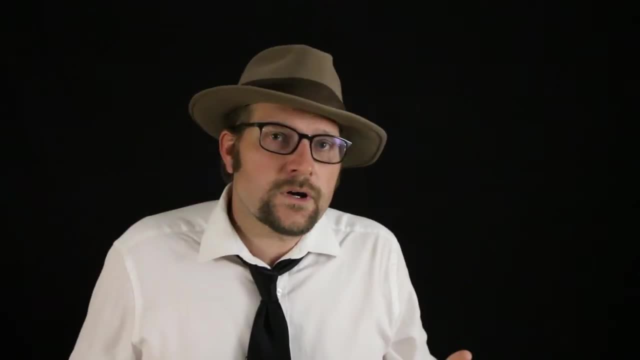 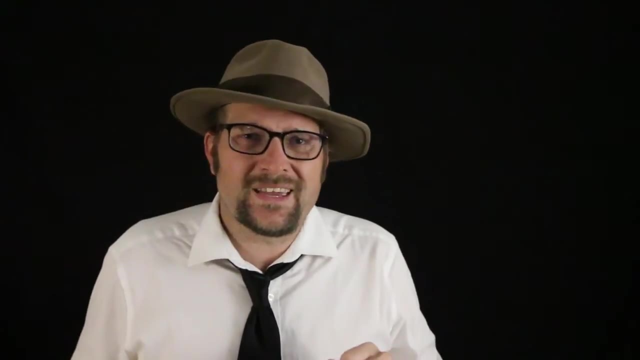 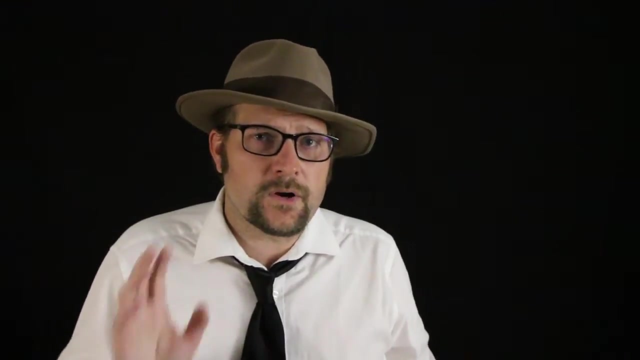 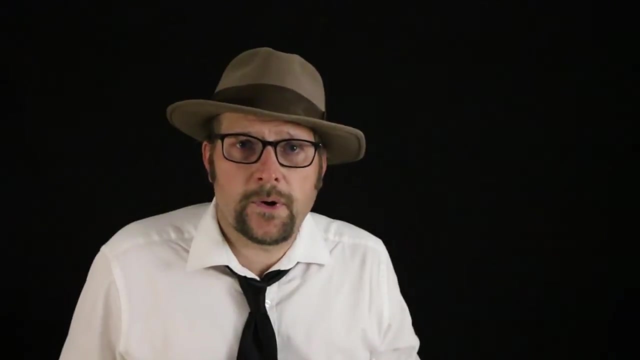 as Velociraptor. The Alitheria were likely egg-laying mammals like modern monotremes, but exhibit an epic pubic bone like marsupials, and so could have been a pouched animal like modern marsupials. No fossil mammal eggs have been found in the Mesozoic The epipubic bone. 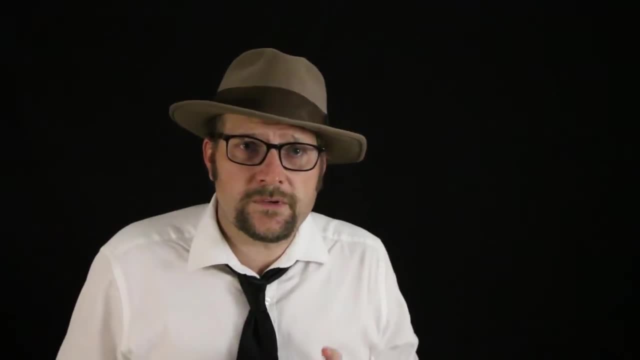 is an extra bone that extends from the pubis bone and supports the body. The epipubic bone is an extra bone that extends from the pubis bone and supports the bone. The epipubic bone is an extra bone that extends from the pubis bone and supports the. 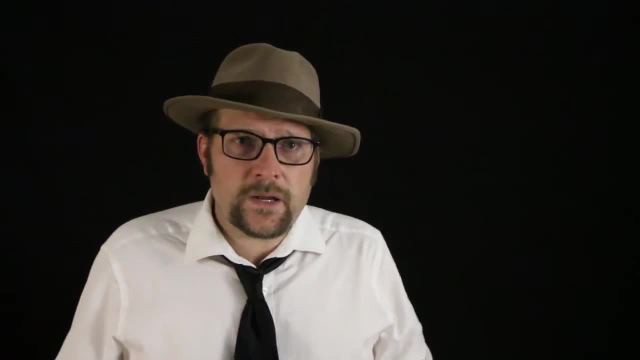 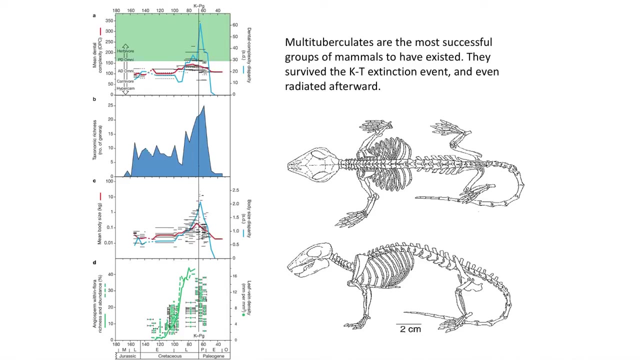 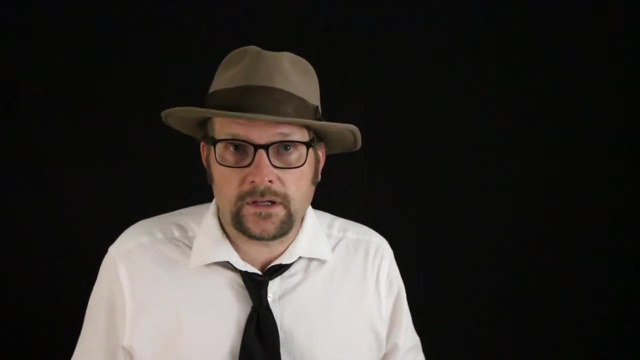 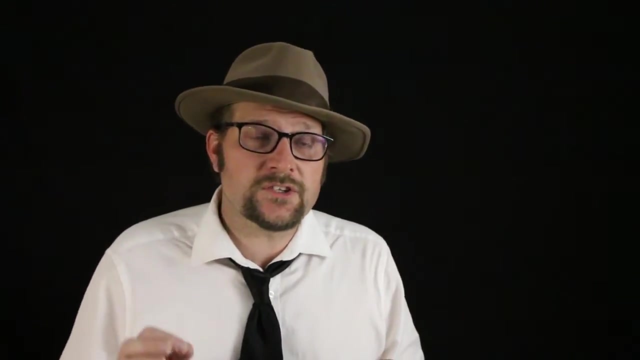 belly, although its function in regard for carrying pouched offspring is unverified. The Multituperculates were highly successful, and it is particularly striking to see their long success, given how many millions of years they lived on Earth. They arose in the early Jurassic and only succumbed to extinction in the early Eocene. 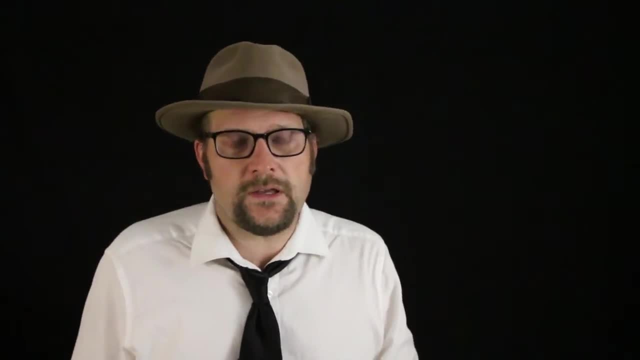 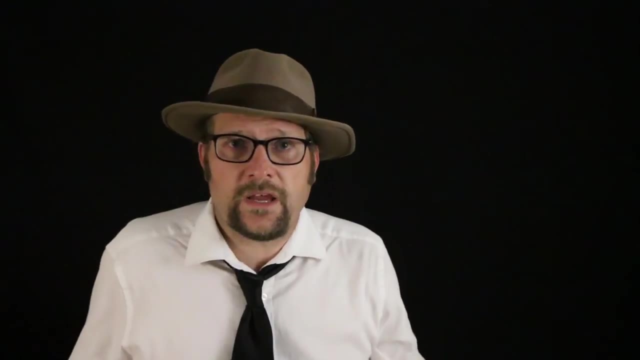 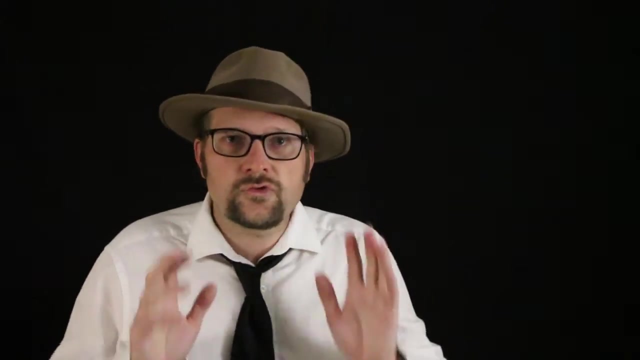 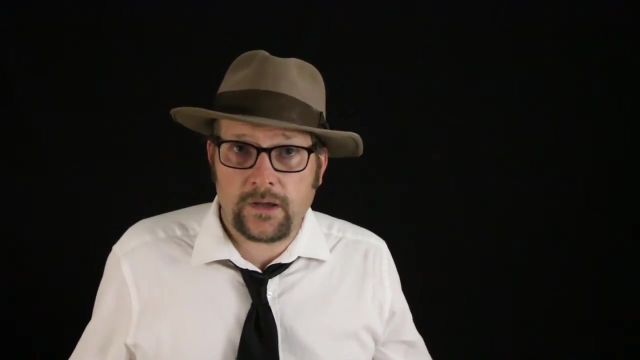 with a run of nearly 150 million years. My own research into their extinction appears to support the idea that climate change associated with the global warming event at the Paleocene-Eocene boundary was extremely detrimental to their survival. Specimens are common in the Paleocene of North America and the Multituperculates are a major component of the Paleocene fauna. However, after the great climatic event at the Paleocene-Eocene boundary, they are extremely rare in the early Eocene, with fewer than 10 occurrences In the Eocene. the rodents which had evolved earlier during the Paleocene were able to. exploit the recovered forests of the early Eocene from this abrupt period of hot temperatures that burned off the great forests with fires. at the Paleocene-Eocene boundary, Multituperculates were able to survive the K-T boundary, but climate change and the rise 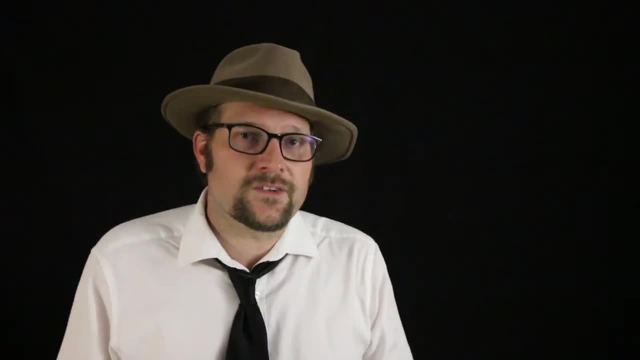 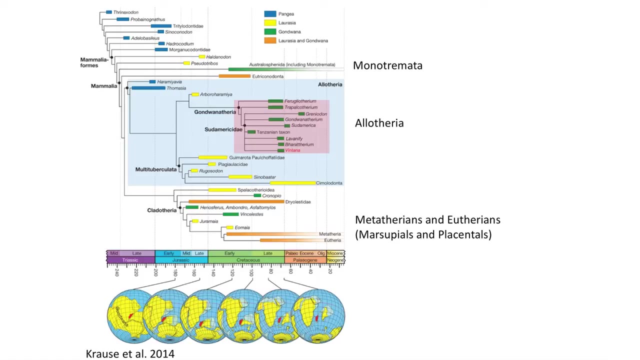 of the rodents doomed the group to eventual extinction. Another group of Alatheria to mention are a group likely related to the Euhyramibeidae, but are restricted to the southern continents during the Cretaceous, the Gonwanatheria. 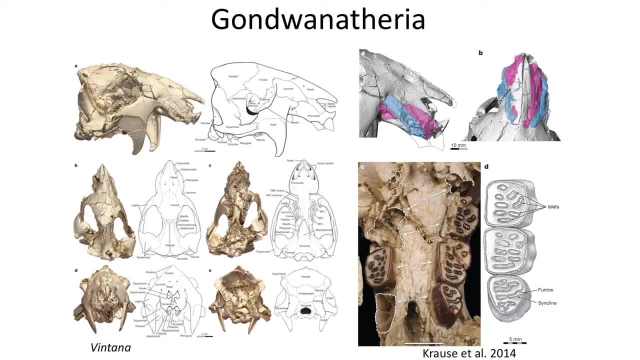 known mostly from isolated teeth. The best-known Gonwanatheria is Ventana, from Madagascar. It was a marmot-like mammal with multicust molars that show quite a bit of wear from chewing, like modern grinding mammals, and large prokumbent incisors. 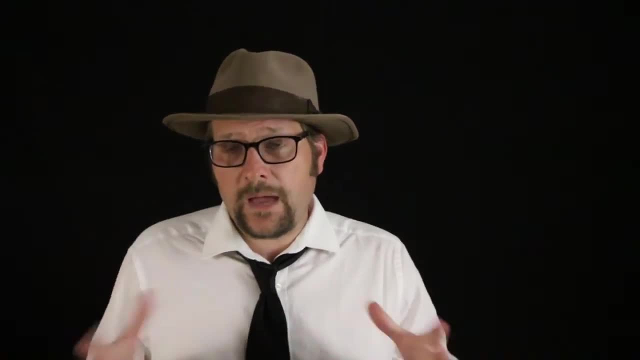 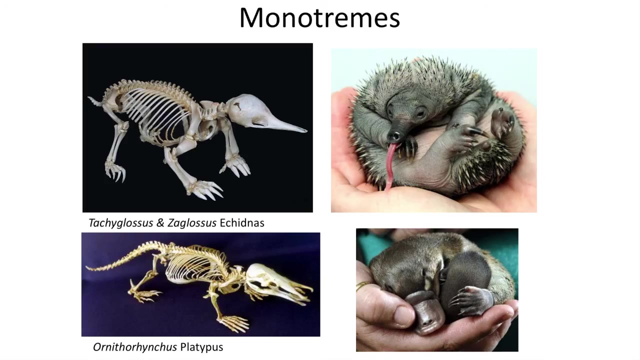 Often depicted as the first or second branch on the mammal tree are the monotremes, a group that includes three lobes. There are three living genera, Tachyoglossus and Zyglossus, the echidnas found in Australia. 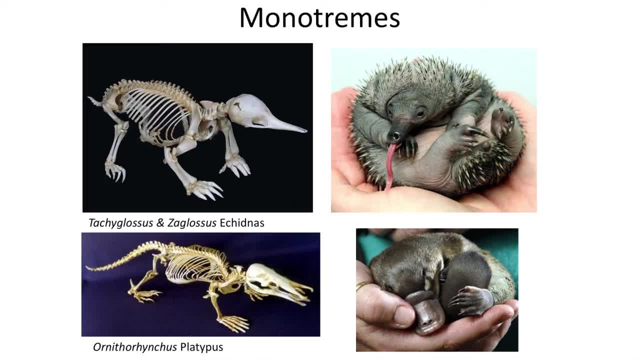 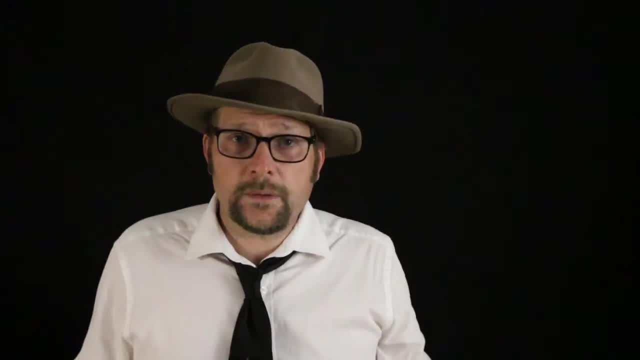 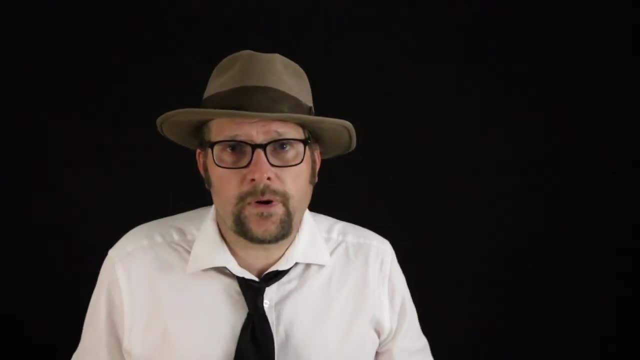 and Tasmania, and Ornithorhynchus, the platypus found in the rivers along the east coast of Australia. Monotremes lay eggs, and hence, when they were first discovered, they were quickly realized to belong to a primitive group of mammals called the monotremes. 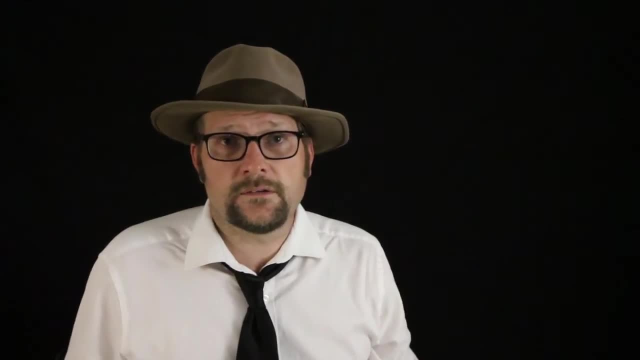 Monotremes and several known multituperculate phytoplankton. Monotremes are the only specimen of a species that can be identified as a living species. Monotremes and other fossil skeletons exhibit bony spurs on their ankles in male individuals. 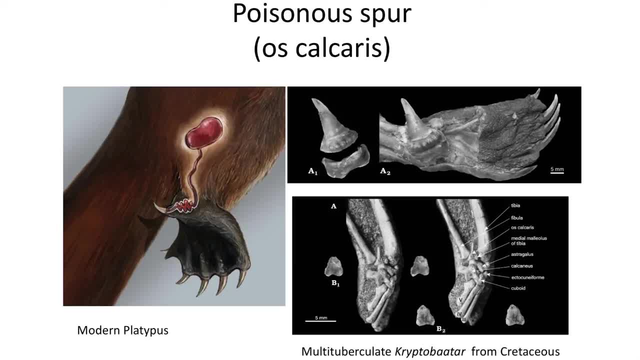 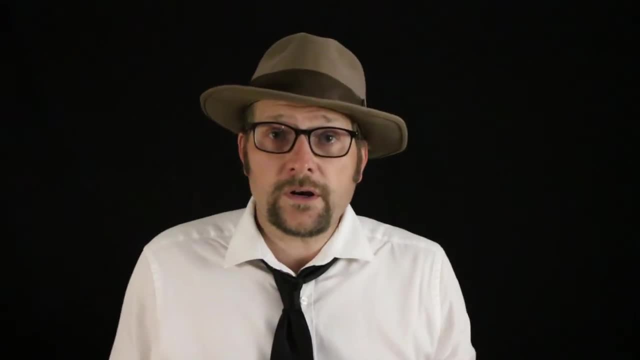 In the living platypus. these spurs connect to a poisonous gland which injects venom and is thought to play a role in interspecies competition during the breeding season, and was likely found in the common ancestor of both groups. The fossil record of monotremes, however, is rather patchy. but is quickly diversifying, with new discoveries During the Late Jurassic and Cretaceous. two groups are often placed within the Monotremata group: the Eutrichonodonta, which includes a range of mammals united by having three cusps on their teeth, and the Ostreosphenidae, a small group that is limited to Australia. 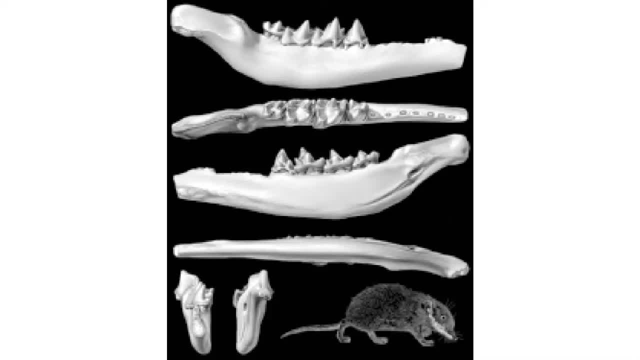 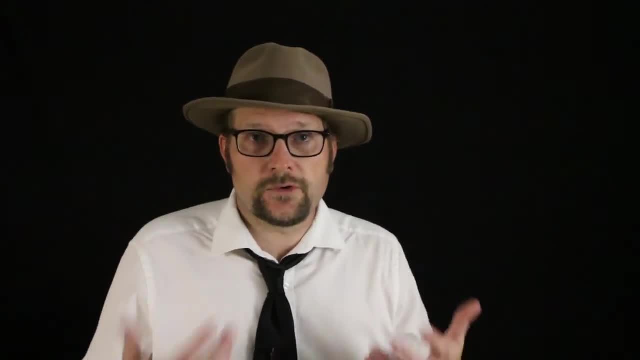 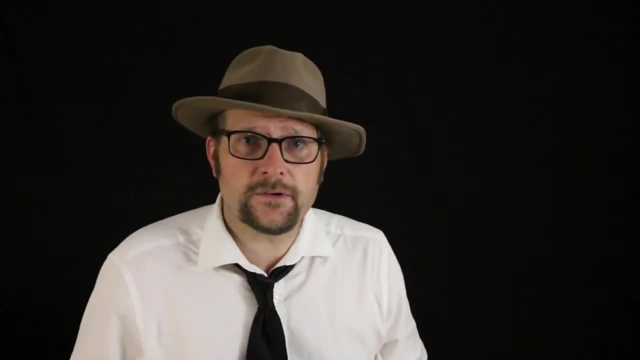 South America and Madagascar, which exhibit a weirdly looking tribosphenic molar. Alright, you should be able to distinguish the unique traits found in the multituberculates, the Alatheria, such as their prokumbent incisors, multicast teeth, bony ankle spurs and their 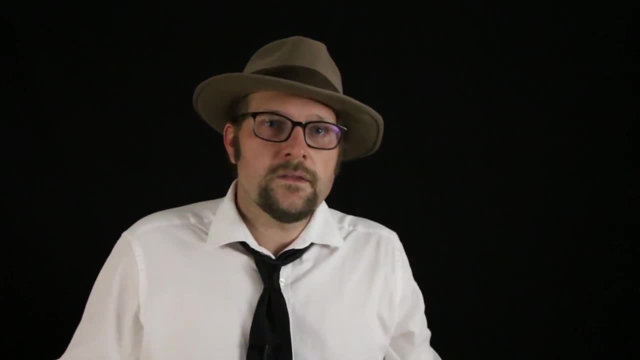 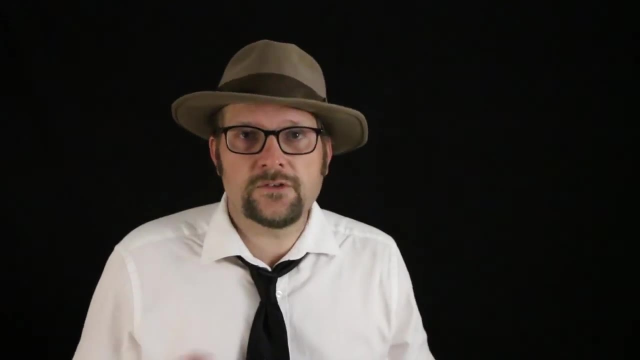 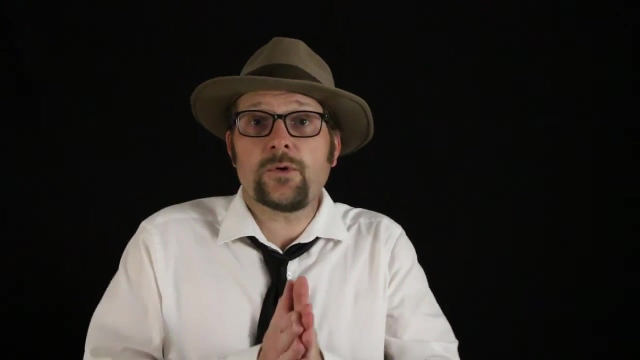 relationship to modern monotremes. In the next video, I will teach you about the tribosphenic molar and introduce you to the Osbornean terminology. Thank you for watching. If you would like to learn more about Utah State University's geology program, check.